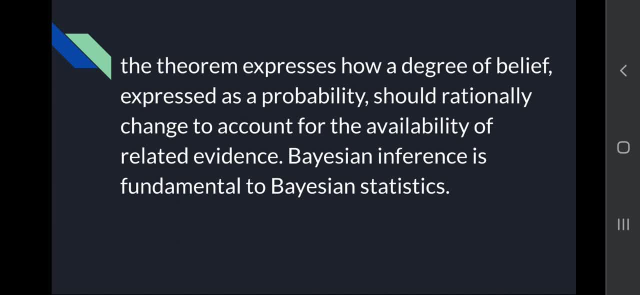 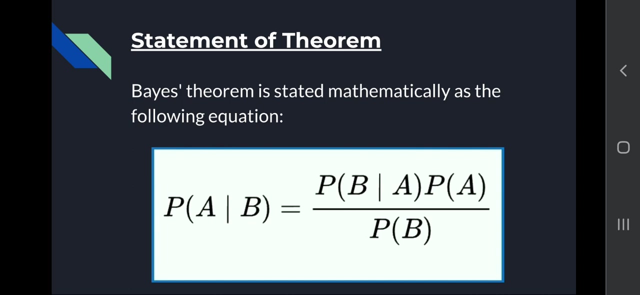 of belief expressed as probability should rationally change to account for the availability of related evidence. Bayesian inference is fundamental to Bayesian statistics. Statement of Theorem. Bayes' theorem is stated mathematically as the following equation: Mortal, proved probability of fact correct. 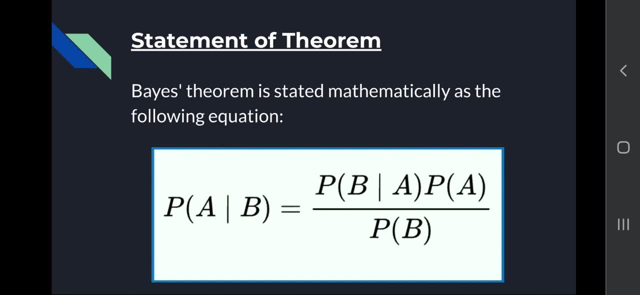 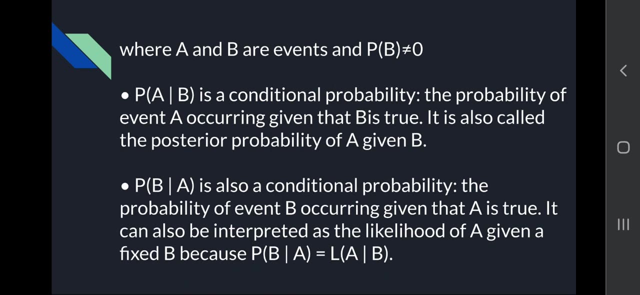 to P. div. P of A by B is P of B by A into P. here is P of A by P. here is known as P of P. and probability of B is not equal to zero because if probability of B equal to zero it goes into undefined. Probability of A by B is a conditional probability. The probability 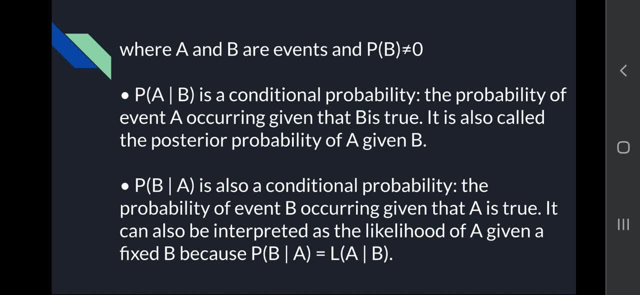 of event A occurring given that B is true. It is also called the posterior probability of Senator A given P. The probability of B by A is also a conditional probability. The probability of event B occurring given that A is true can also be interpreted as the likelihood of. 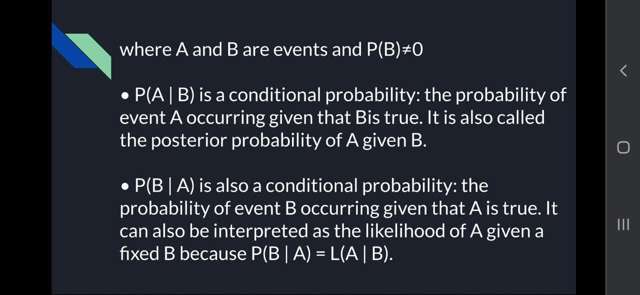 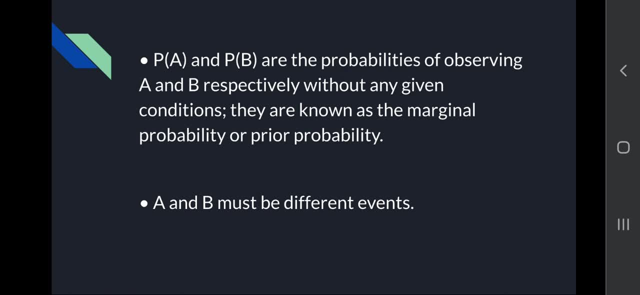 A given fix B. The best probability of B by A is a constant probability. This probability can also be equal to l of a by b. Probability of a and b are the probabilities of observing a and b respectively without any given conditions. They are known as the marginal probability, or 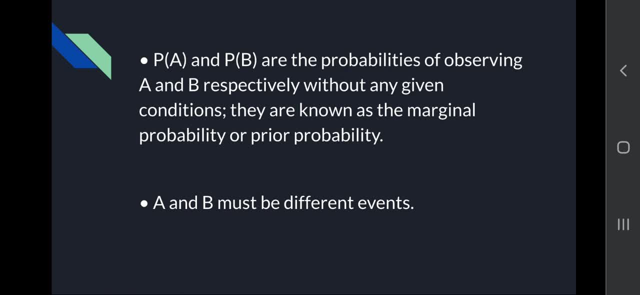 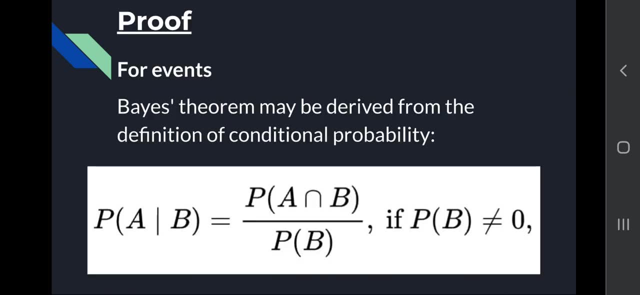 prior probability. a and b must be different events. They cannot be same events. proof of the theorem For events- Bayes theorem- may be derived from the definition of conditional probability. Here, the definition of conditional probability is that probability of a by b is always equal to l of a by b. Probability of a by b is always equal to l of a by b. Probability of 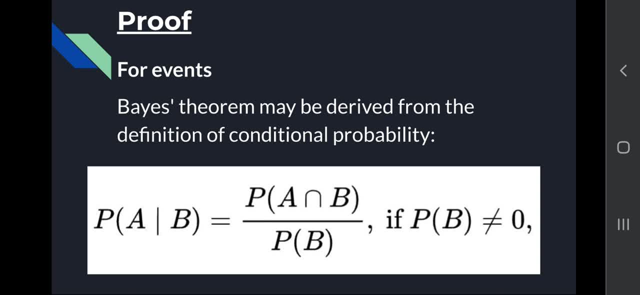 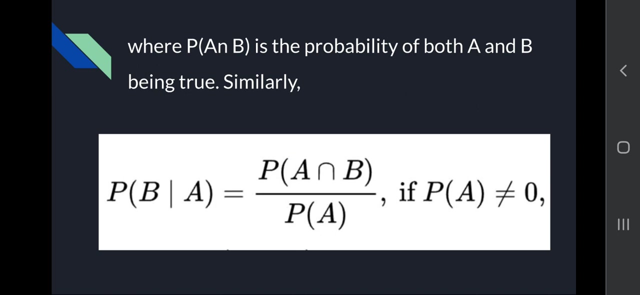 a by b is always equal to probability of a intersection b divided to probability of b, only if probability of b is not equal to zero. That means that probability of b is should not be equal to zero Where probability of a intersection b is the probability of. 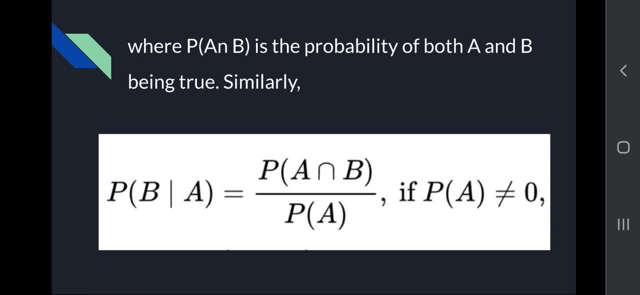 both a and b being true. Similarly, probability of B by A is always equal to probability of A. intersection B: 2 divided by probability of A and the probability of A should not be equal to 0. It means that the probability of A value should not be equal to 0 in any space. 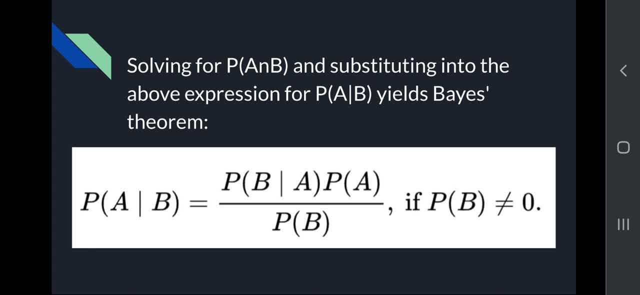 Solving for probability of A intersection B and substituting into the above expression for probability of A by B yields Bayes theorem. Here we can see that probability of A by B is equal to probability of B by B, B by A into probability of A whole divided by probability of B and here probability of. 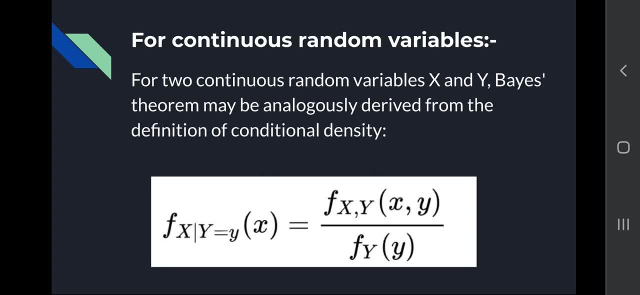 B is not equal to 0.. For continuous random variables: for 2 continuous random variables, x and y, Bayes theorem may be analogously derived from the definition of conditional density. Here we can see that B by B is equal to 0 and A is equal to 0. 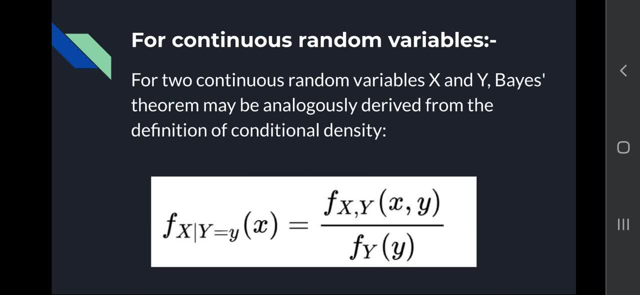 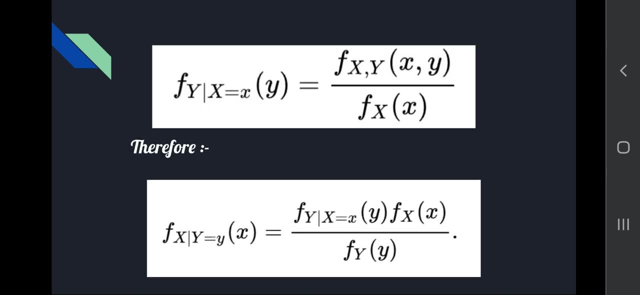 f of x by y is equal to y to the power of x is equal to f of x comma y brackets x comma y by f of y into y, We can. and another one would be f of y by x, similarly to the previous one, that was.